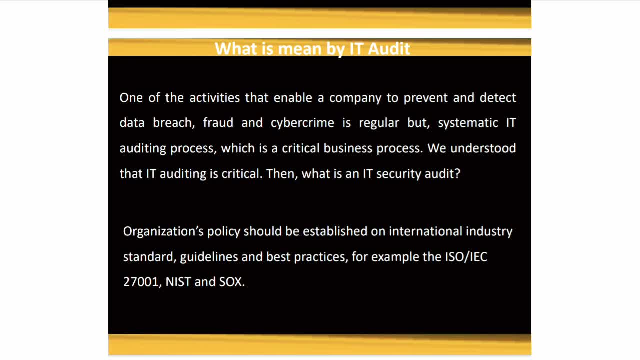 cybercrime is a regular but systematic IT auditing process, which is a critical business process. We understood that IT audit is critical. Then what is an IT security audit? Organization policy should be established on our international industry standards, guidelines and best practices. We have to already learn the ISO IES to 27001 standard, NIST and ISO X So. organization policy should be established on our international industry standards, guidelines and best practices. We have to already learn the ISO IES to 27001 standard, NIST and ISO X So. organization policy should be established on our international industry standards, guidelines and best practices. We have to already learn the ISO IES to 27001 standard, NIST and ISO X So. organization policy should be established on our international industry standards, guidelines and best practices. We have to already learn the ISO IES to 27001 standard, NIST and ISO X So. organization policy should be established on our international industry standards, guidelines and best practices. We have to already learn the ISO IES to 27001 standard, NIST and ISO X So organization policy. 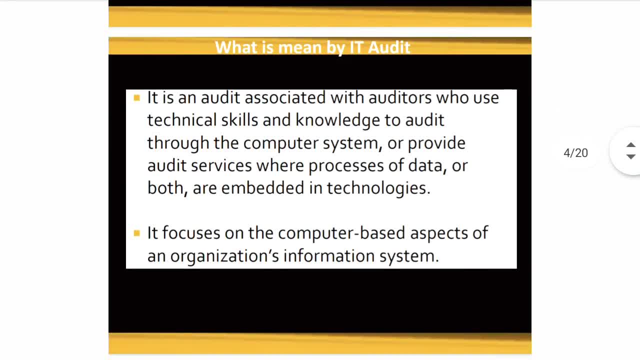 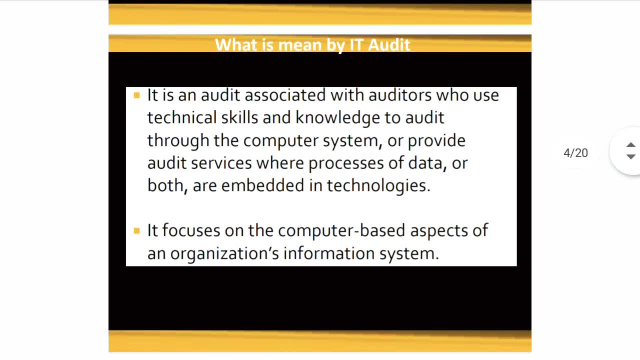 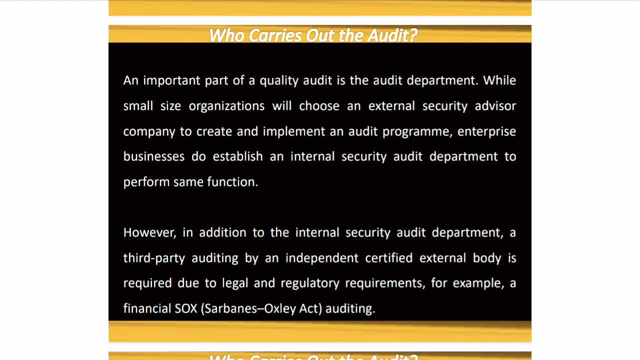 Now let's see. it's a firm, that is, a who carries out the audit. An important part of quality audit is the audit department. the department will functioning separately, while a small size organization will choose an external security advisor and company to create and implement an audit program. 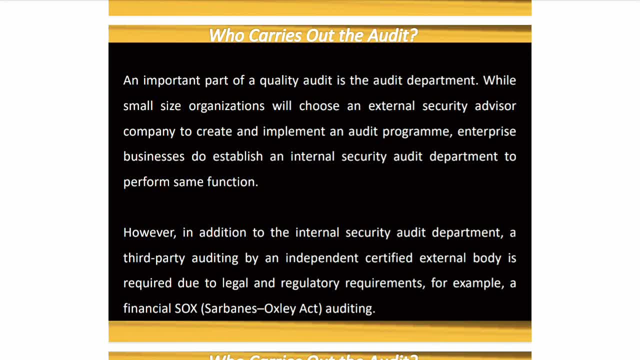 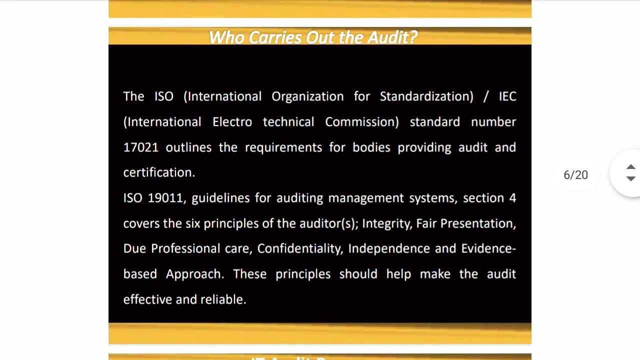 Enterprise businesses do establish an internal security audit department to perform the same functions separately. However, in addition to the internal security audit department, a third party auditing by an independent, certified external body is required due to legal and regulatory requirements. So the ISO is one of the organization that will be an international organization for 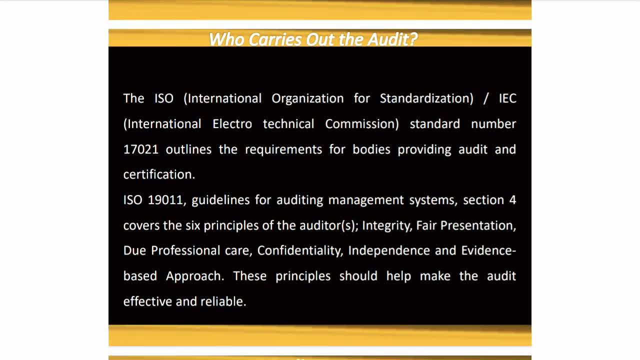 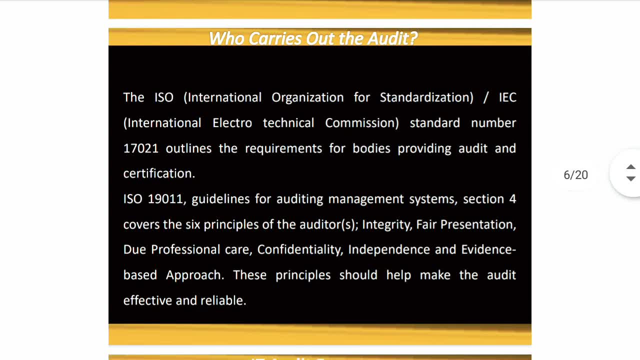 standardization, IES. that will be International Electro-Technical Commission. standard number will be 17021 outlines. 3. The requirements for bodies providing audit and certification. ISO 19011 Guidelines for Auditing Management System. section 4 will cover the six principles of the auditors that will be very important for the cybersecurity. 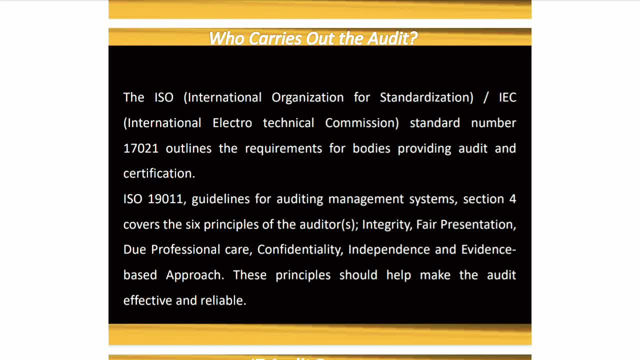 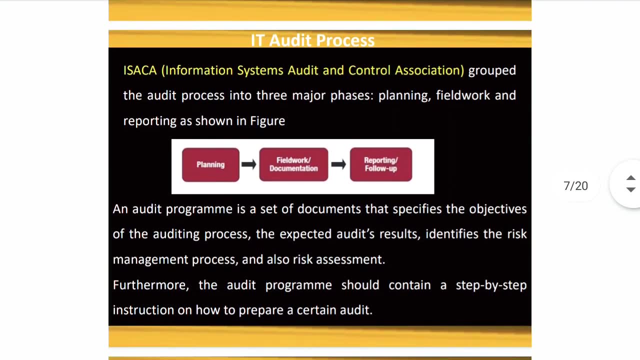 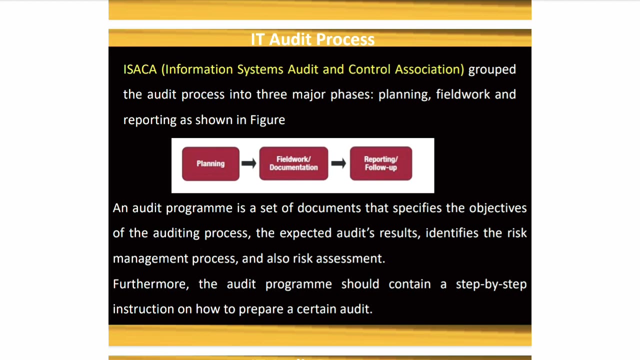 That will be integrity, fair presentation, due professional care, confidentiality, independence and evidence-based approach, and these principles should help make the audit effective and reliable. Now let us have a look on IT Audit Process. It is a very critical process, but it will be mainly divided into three important parts. 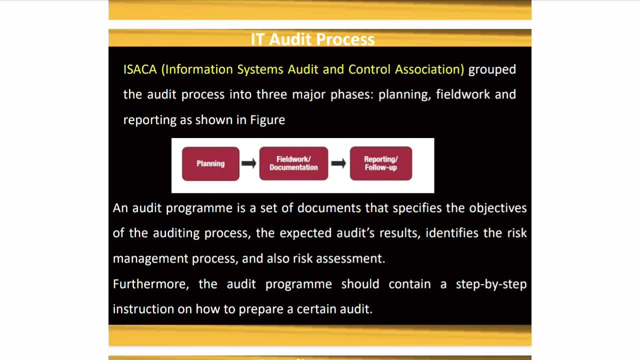 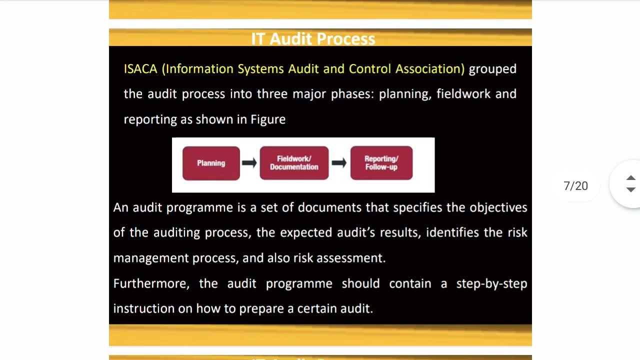 ISACA is one of the organization we called it as a Information Systems Audit and Control Association group. the audit process into mainly three phases: planning, fieldwork and reporting. An audit program is a set of three phases Set of document that specify the objectives of the auditing process, the expected audits. 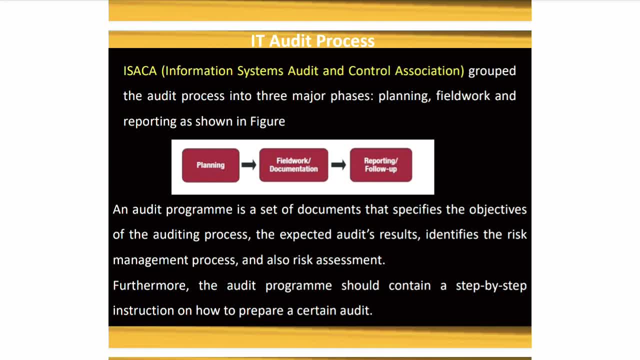 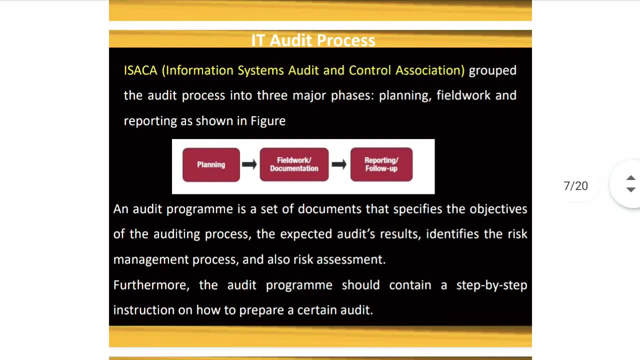 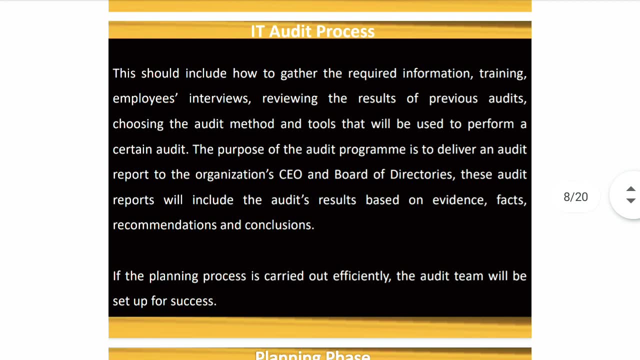 results, identify the risk management processes and also risk assessment. Furthermore, the audit program should contain a step-by-step instruction on how to prepare a certain audit. This should include how to gather the required information, training and employees interviews, reviewing the results of previous audits, choosing the audit method and tools that will 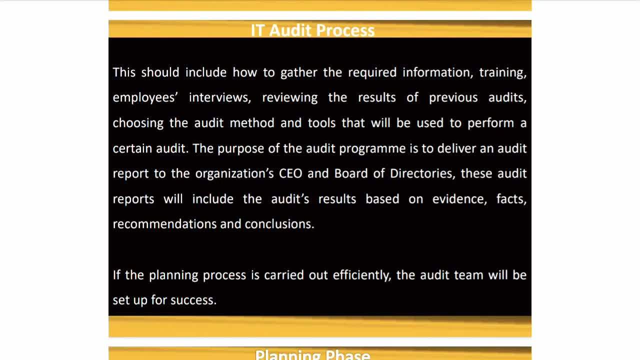 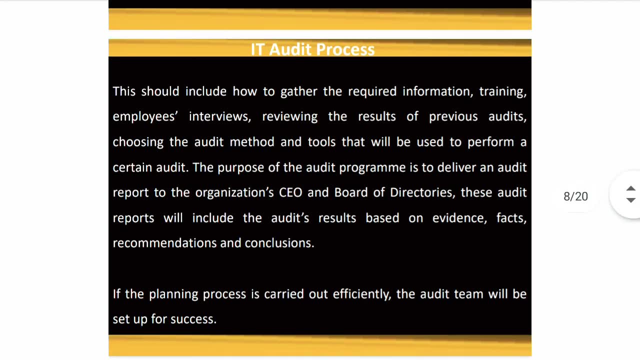 be used to perform audits. The purpose of the audit program is to deliver an audit report to the organization's CEO and Board of Directors. These audit reports will include the audit's results based on evidence, facts, recommendations and conclusion. If the planning process is carried out efficiently, the audit team will be set up for the success. 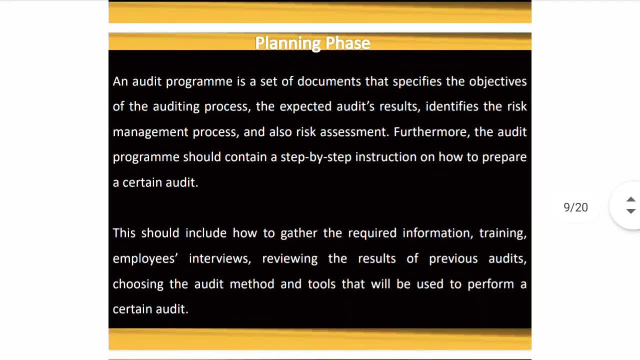 So, in the particular audit phase, the first important phase is the execution of the audit audit phase. first important phase is the planning phase. an audit program is a set of documents that specifies the objectives of the auditing process, the expected audits results, identifies the risk management process and also risk assessment. furthermore, the audit program should: 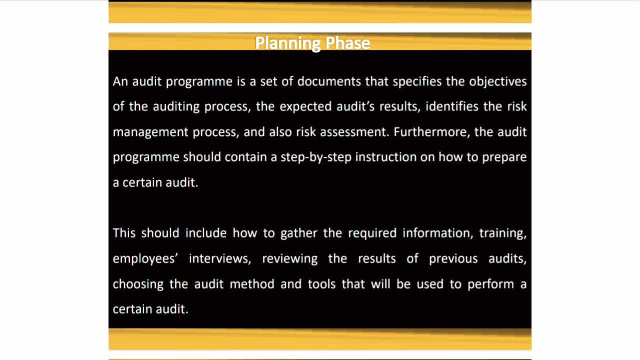 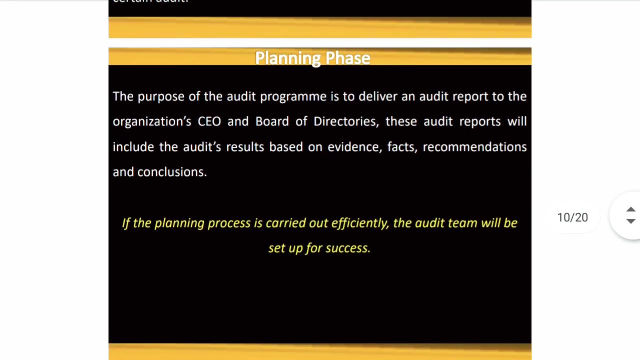 contain a step-by-step instruction on how to prepare a certain audit. this should include how to gather the required information, how to provide training to the employees, how to conduct interviews, how to review the results of previous audit, and choosing the best audit method and tools that will be used to perform a certain audit. the purpose of the audit program. 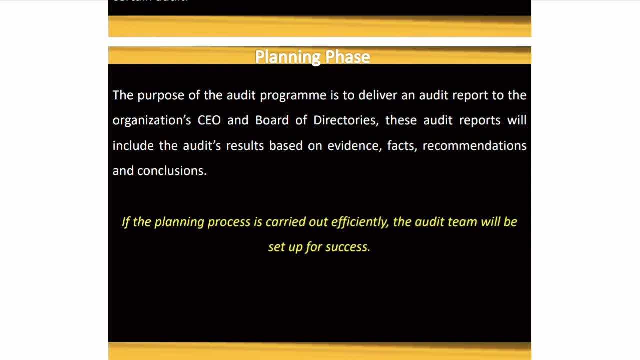 is to deliver an audit report to the organization's CEO and board of directors, and these audit reports will include the audits results, best on evidence, facts, requirements and the required procedures for the audit process and the mistakes that the auditors can make and how you can. If the planning process is carried out efficiently, the audit team will be set up for the success. 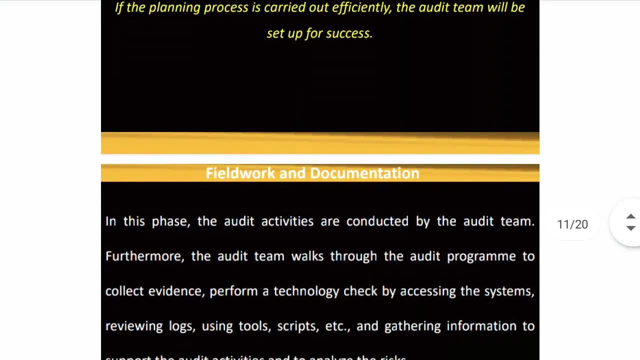 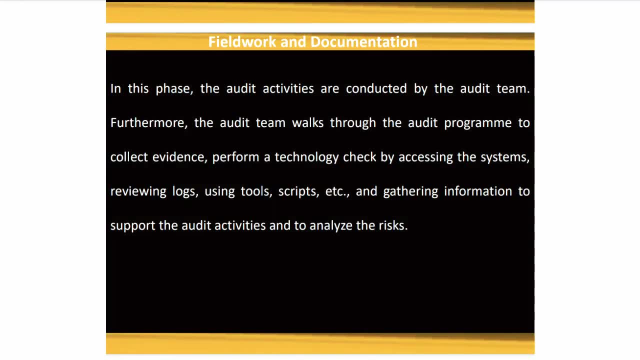 Hence it is a very important phase in the audit process. Second important phase is the field work and documentation. In this phase, the audit activities are conducted by the audit team. Furthermore, the audit team walks through the audit program to collect evidence, perform. 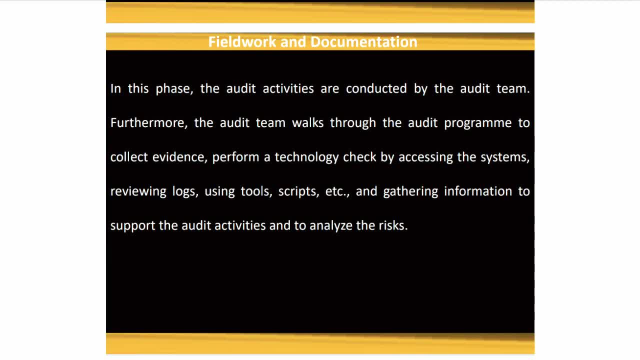 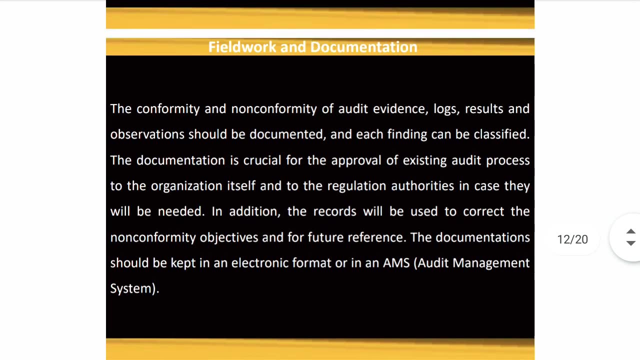 a technology check by accessing the systems, reviewing the laws, using the tools, scripts and gathering information to support the audit activity and to analyze the risk. The conformity and non-conformity of audit evidence, log results and results are documented. 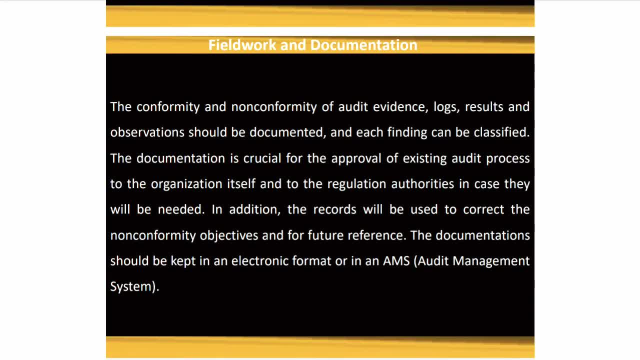 and each finding can be classified. The documentation is crucial for the approval of the existing audit process to the organization. In addition, the records will be used to correct the non-conformity objectives and for future reference. The documentation should be kept in an electronic format or in an AMS system. 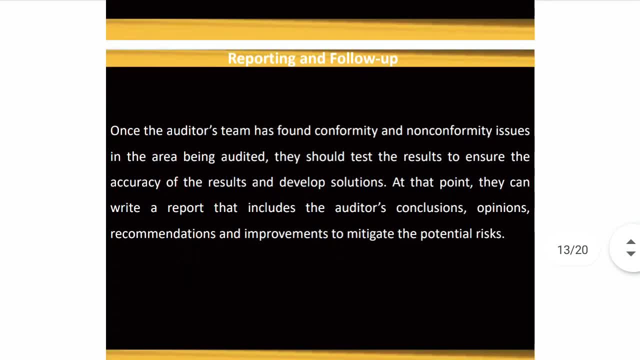 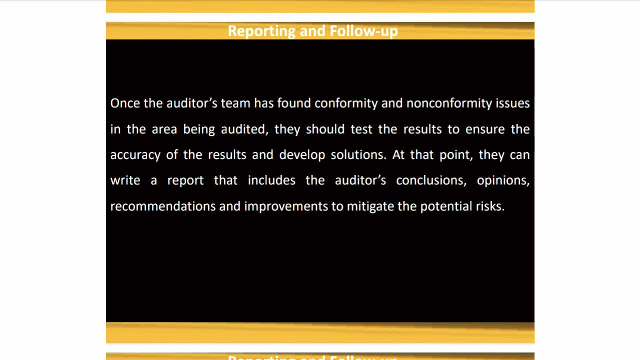 Third important step will be the reporting and follow-up. That is, everything will be kept in the form of documentation. Once the auditor's team has found conformity and non-conformity issue in the area being audited, they should test the results to ensure the accuracy of the results and develop the 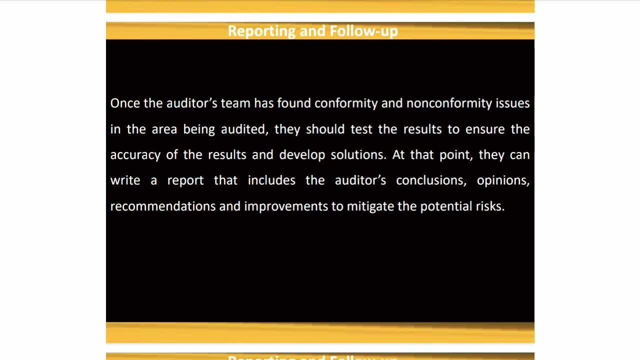 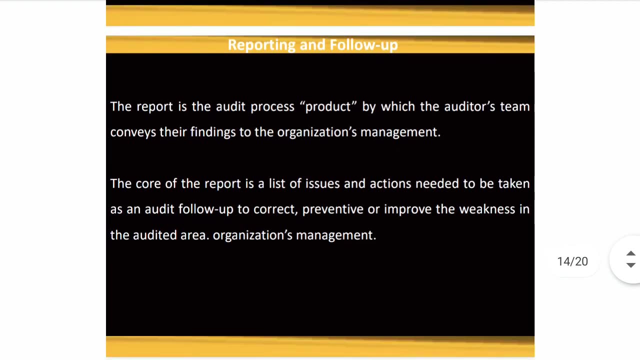 solutions. At that point they can write a report that includes the auditor's conclusions, opinions, recommendations and improvements to mitigate the potential risk. The report is the audit process That will be a product By which the auditor's team conveys their findings to the organization management. 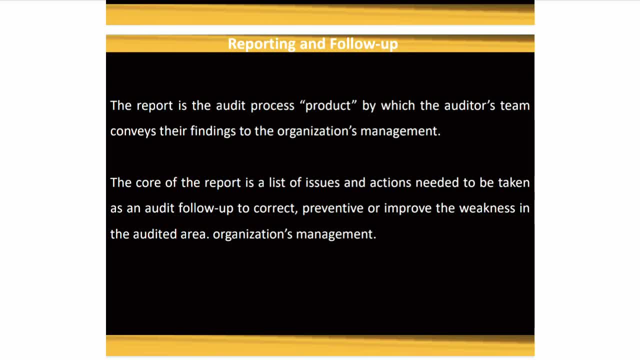 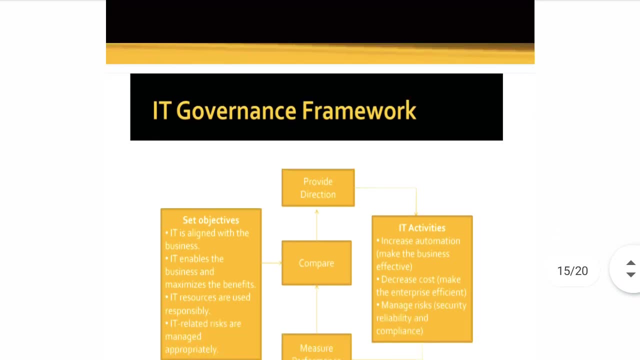 The core of the report is a list of issues and actions needed to be taken as an audit follow-up to correct, prevent or improve the weaknesses in the audited area: organization management. So it will be the full opening of the organizational functioning. 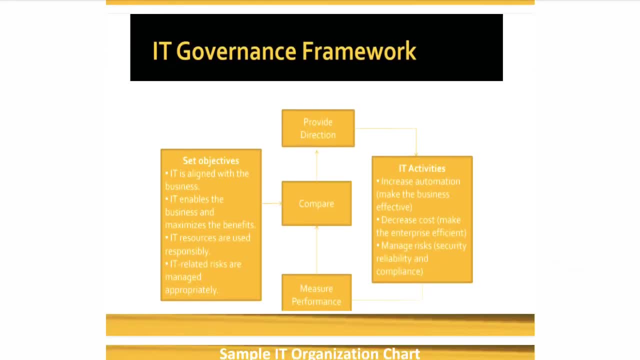 Now let us have a look on the IT governance framework. It is one of the very important IT organization or framework will provide the guidance to the particular organization. Basically, the particular organization has. any IT organization has set their objectives, That is, IT is aligned with the business. 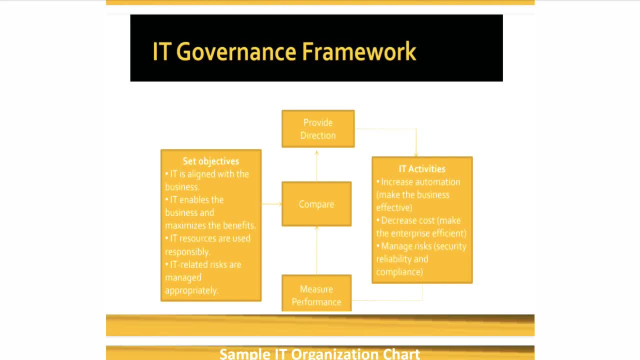 IT enables the business and maximize the benefits. IT resources are used responsibly and it relates to risk- are managed appropriately. Now let's see the next step. Now, particular IT governance will provide the direction to the organization and define IT activities. That is, increase the automation, decrease cost. 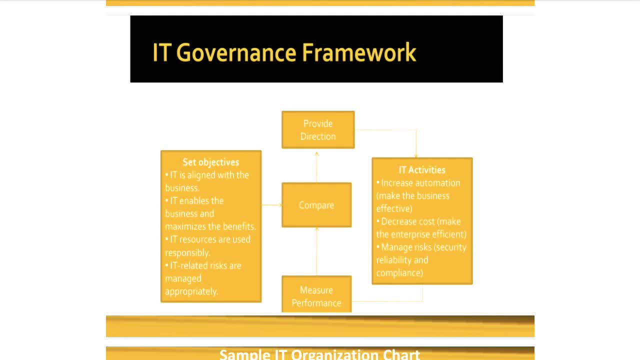 It will be make the business effective. It will be make the enterprise efficient and manage the risk to provide the security, reliability and competency to the organization. Now, through this defined IT activities and particular set objective, IT will be able to manage the risk. 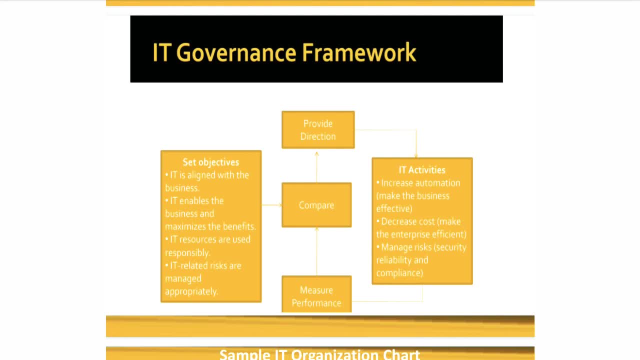 IT governance will measure the performance of the organization and they will compare that performance with the set objectives and define IT activities. and that particular direction has been provided by the IT governance And hence in every organization, if there is a successful governance, then definitely. 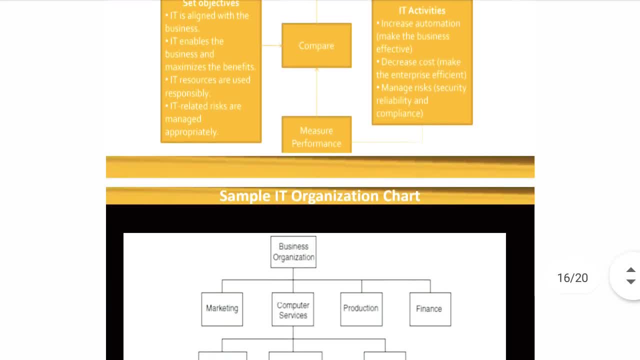 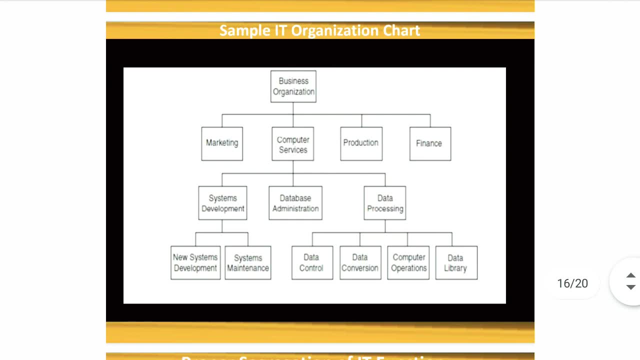 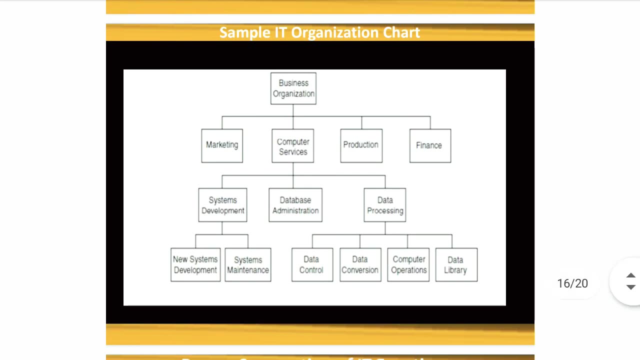 organization will manage the all activities efficiently. Now this is one of the sample of IT organization chart. Any business organization has a different departments, mainly the marketing, computer services, production, finance. computer services has divided into three different important aspects. that will be system development, database administration, data processing. 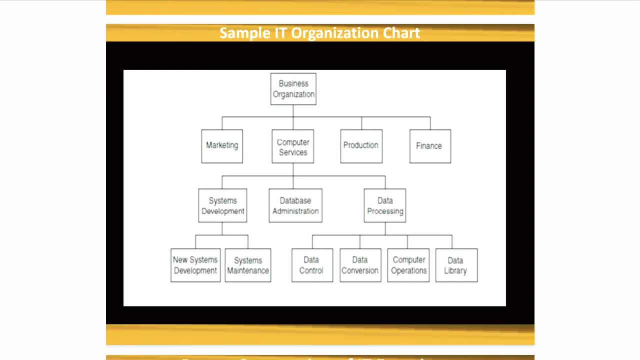 and in the cyber security we require the system development that will be the new. We have to develop the new system or we have to do the maintenance of the original system In the data processing, One thing that we have to be aware of. 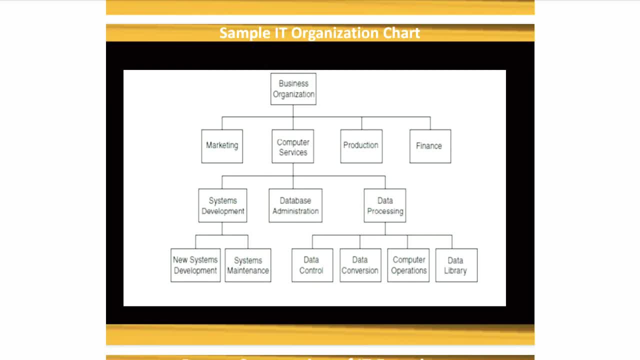 We have to be aware of. One aspect has been required to focus on the organization is the data control, data conversion, computer operations and data library. So these two aspects has been work under the computer services to give the maximum beneficial services to the organization. 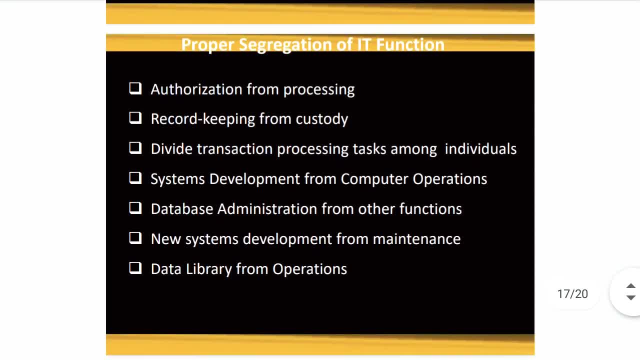 Now the here is a segregation of IT function. IT function or IT authority has been segregate their particular duties. that will be the authorization for the organization, The systems that they have to segregate their duties. This is called redevelopment from operations. The data is set aside for the organization that will be the first to be been segregated. 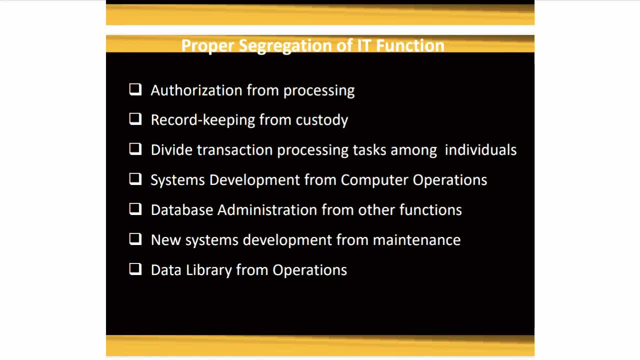 from the organization. The system evaluation needs to be done to define, based on the customer's needs, and we have to be clear on this concept. That is why we are using their name. Now, data library has been segregated from processes So, according to that, IT department has segregated their duties. 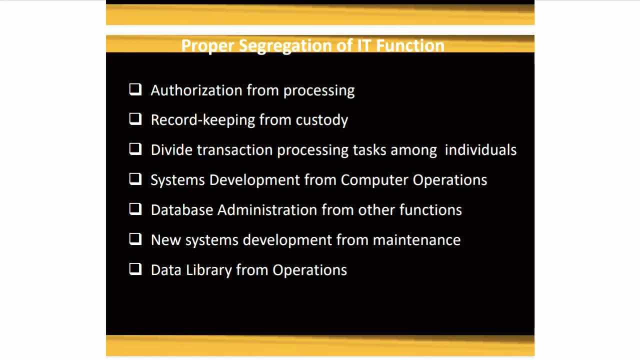 Now let's see what other functions have been done in the previous system. This is the same process in the previous system. This is where the degeneration of the organization has been done. The system has been divided into three main do not ど on the other side. 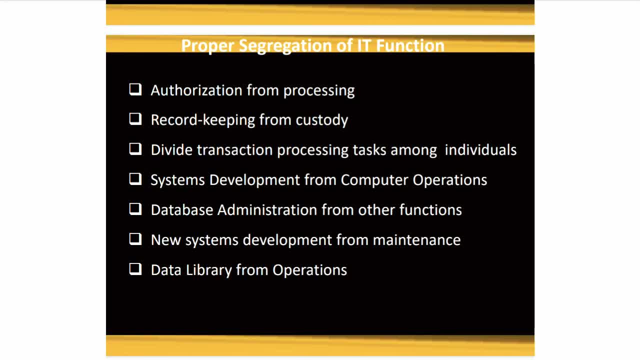 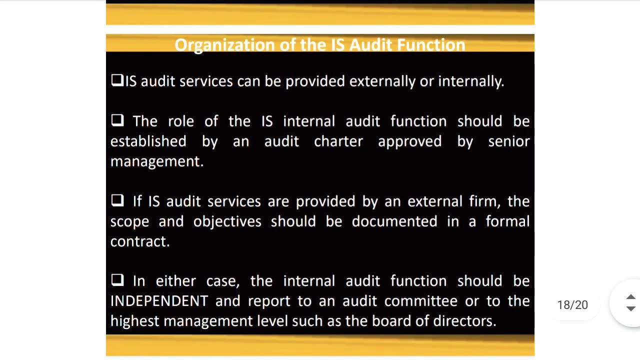 Now let's look at the actions There have been. consists of the three parts of the organization that has been segregated from the organization: development from maintenance, data library from operations. so according to that IT department has segregate their duties. here is the list of audit. 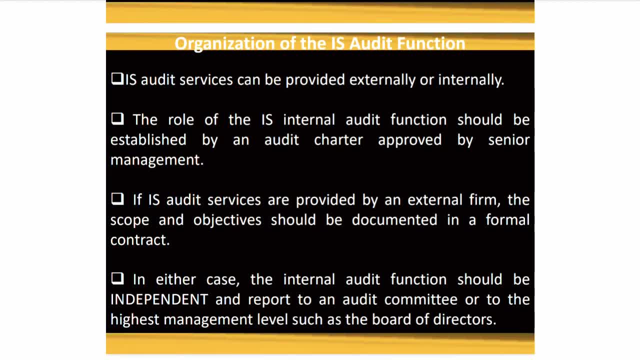 function has been performed by the particular organization. I see our particular is audit services can be provided externally or internally by any of the organization organization had choose any one of the media or both has been implemented in the organization. the role of the is internal audit function should be established by an audit charter approved by the senior. 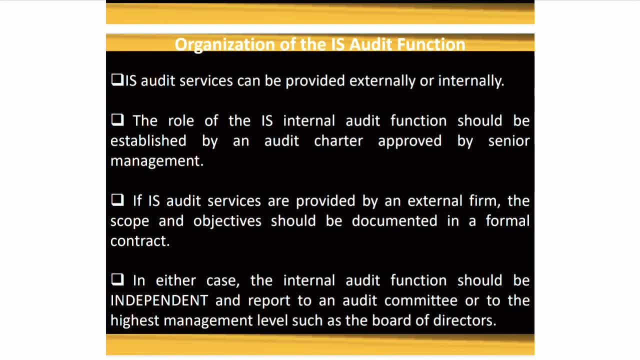 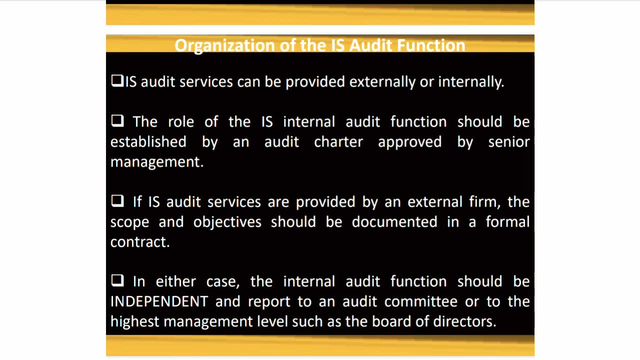 management. if is audit services are provided by an external firm, the scope and objective should be documented in a formal contract. in either case, the internal audit function should be independent and report to an audit committee or to the highest management level, such as the board of directors. here is the list of other functions. actually, all functions should be. 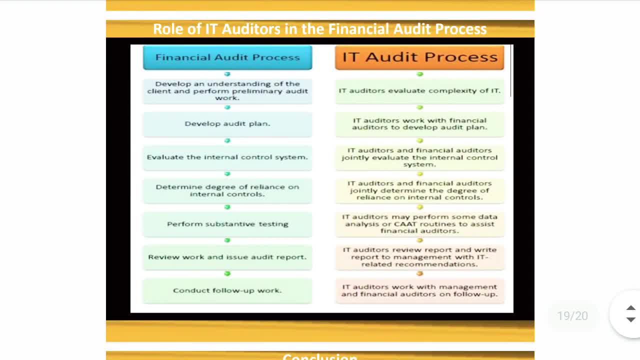 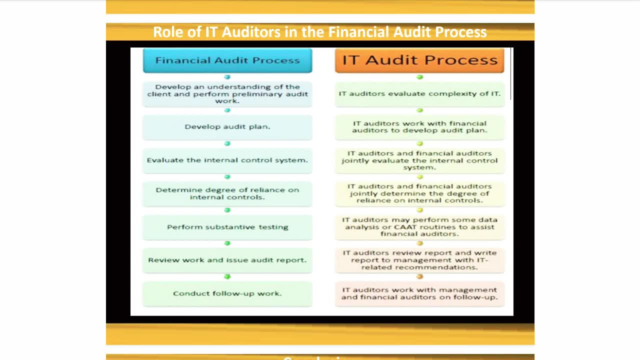 Here is the role of IT auditors in the financial audit process. Normally, you all are aware about the financial audit process. We have to compare this process with the IT audit process. In the financial audit process, basically, we are developing an understanding of the client and perform the preliminary audit work. 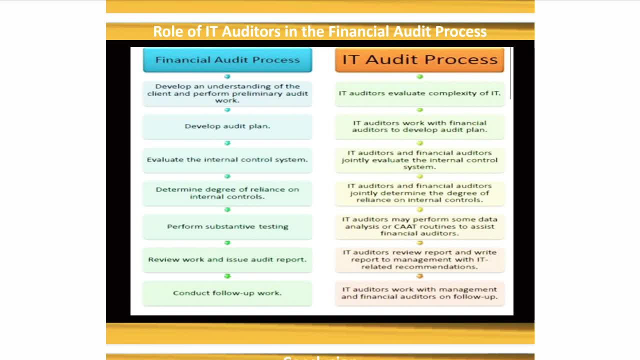 Then we develop the audit plan. After developing the plan, evaluate the internal control system, Determine the degree of reliance on internal controls, Perform the substantive testing, Then do the review work and issue audit report And finally conduct the follow-up work. 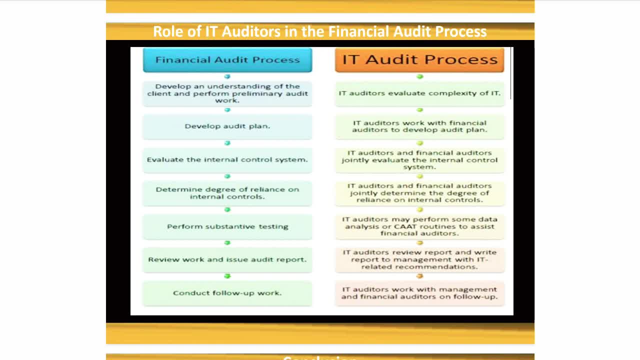 This is happening in the normal financial audit process. Now IT audit process is somewhat different from this process. In IT auditors evaluate complexity of IT That will be the lacuna, or particular lacuna, of the system. IT auditors work with the financial auditor to develop audit plan. 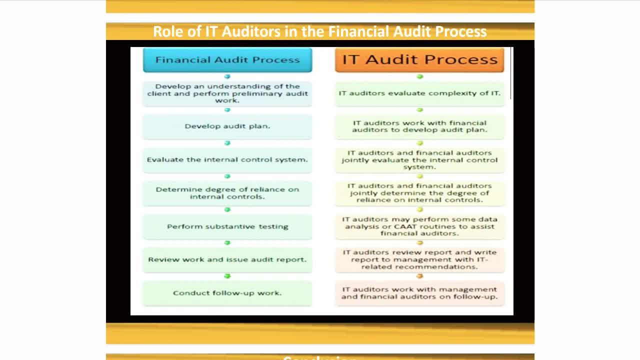 IT auditors and financial auditors jointly evaluate the internal control system. IT auditors and financial auditors jointly determine the degree of reliance on internal controls. IT auditors may perform some data analysis or get routines to assist financial auditors. IT auditors review, report and write report to management with IT related recommendations. 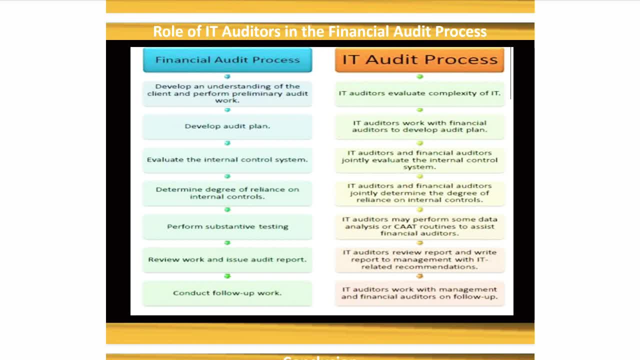 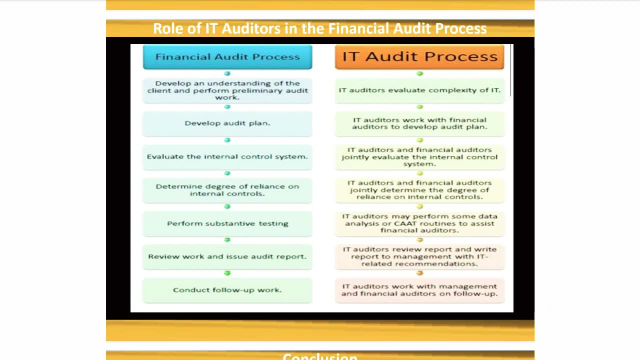 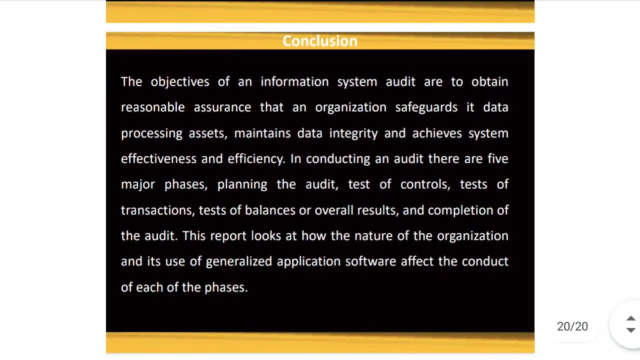 And finally, IT auditors work with the management and financial auditor. And finally, IT auditors work with the management and financial auditors on follow-up to design a beautiful solution or to design the required solution for the problem. And finally, we have to conclude that the main objective of an information system audit are to obtain reasonable assurance that an organization safeguards its data processing assets. 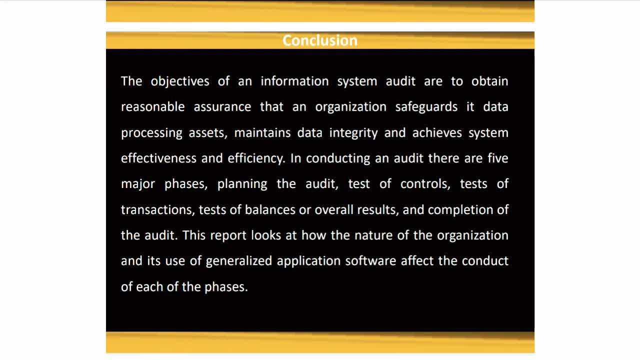 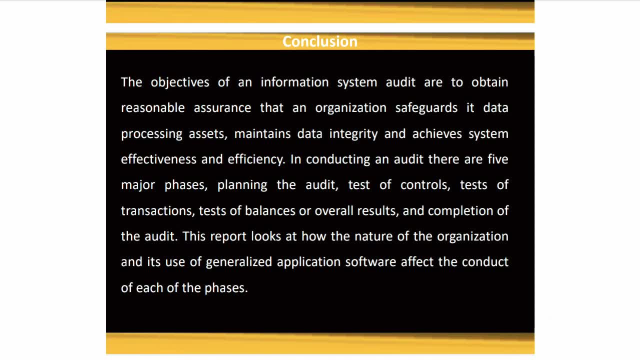 It maintains data integrity and achieves system effectiveness. In conducting an audit, there are five major phases, like the training under an organization and the process of ей, network management and optimizing democracy or performance and who will be the planning of the audit. Test of controls. 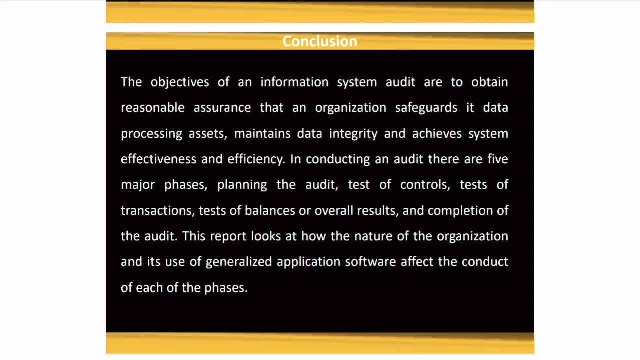 Test of transaction, Test of balances, test of balances or overhaul and completion of the audit. This report looks at how the nature of the organization and it's used and use of generalized application software effect the conduct in each of phases. Heck, those organisations have doing a lot of the organization goals.